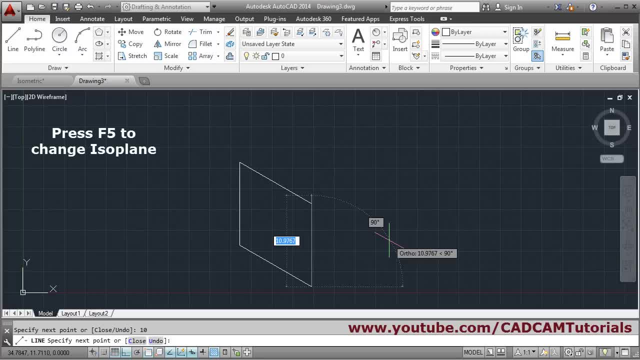 the isoplane you have to click FIU on the keyboard. so press FIU, so when FIU is clicked, plane has been changed. so here is isoplane, top is there and now cursor is going on this side. so using FIU you can change the plane. so as you keep on, 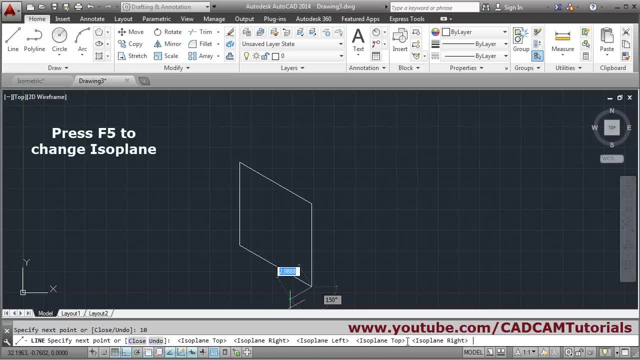 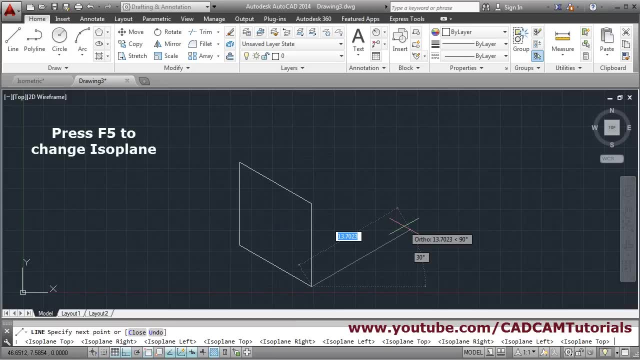 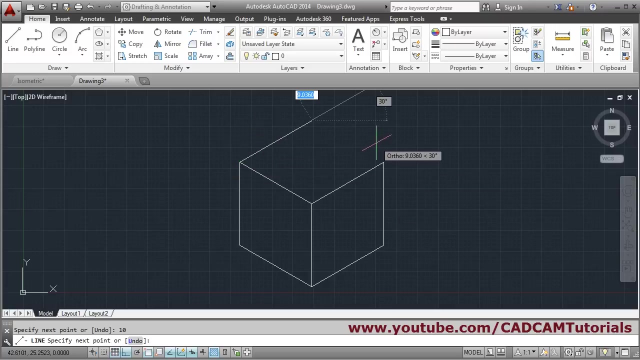 pressing the FIU you can see that the planes are changing here. you can also you directions is changing. so you can by pressing FIU, only so once you got the desired plane you have to stop, then again give the direction and length. then, upper side, I want to draw again line end point again, length again FIU. 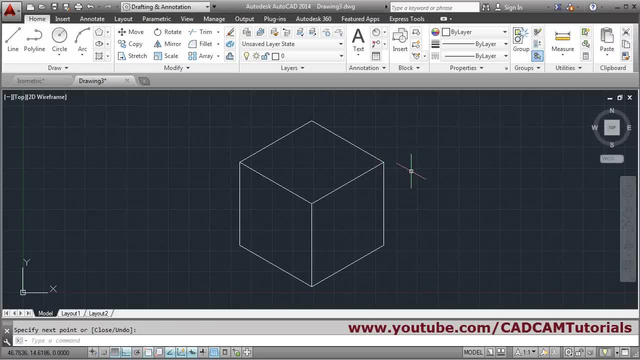 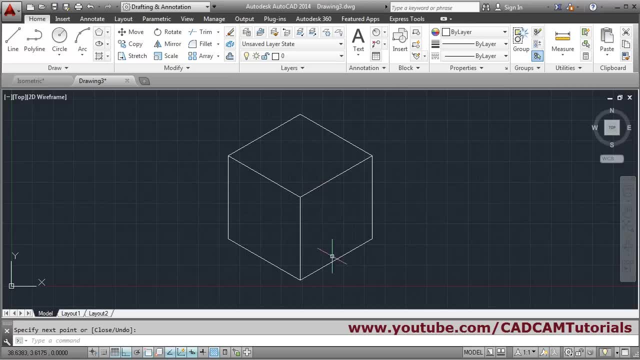 to change the plane and length: enter. to come out now in isometric, offset command is not useful because offset comes straight parallel. but I want to go here, incline in 30 degree inclined. so in place of offset you have to use copy command. so click on copy, select object, enter. 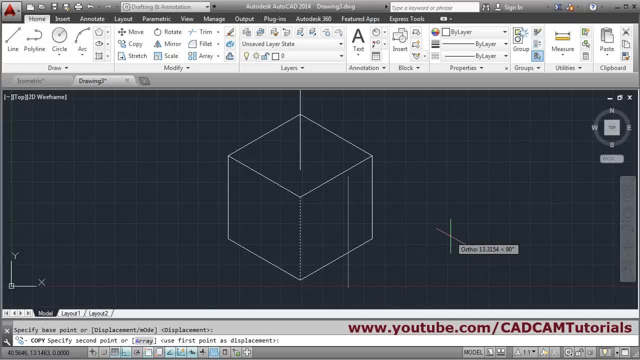 give base point. so I want to go on this side. so again I will press FIU and give direction and give the distance, press ENTER and press ENTER to come out. so in this way you can create offset using copy in isometric. then in isometrics circle is different. so to create a circle you have 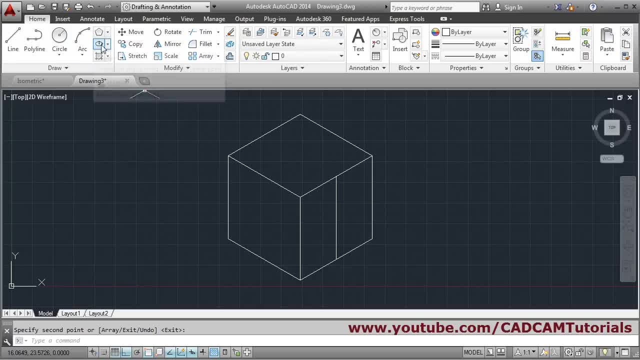 to use axis. you have to use ellipse command, click on the arc and click on axis end point. you have to use axis end command. then, here you can see, one option is added that is ISO circle. so click on that ISO circle option and then click on option and then specify center point for ISO circle, then click the center point. 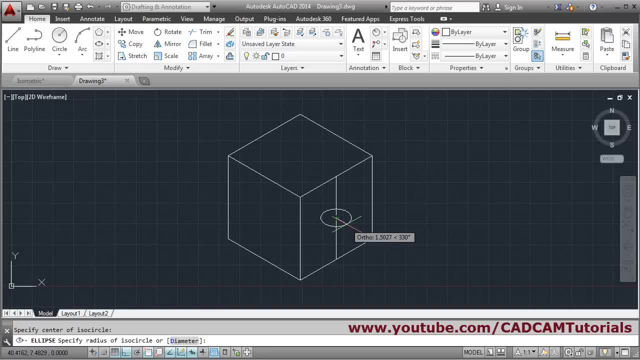 now it is coming in the top plane. so you can change the plane by pressing f5. so you can see that how it is get aligned. once you got the desired location, then give the radius. suppose 5 is the radius. so in this way this isometric circle is: 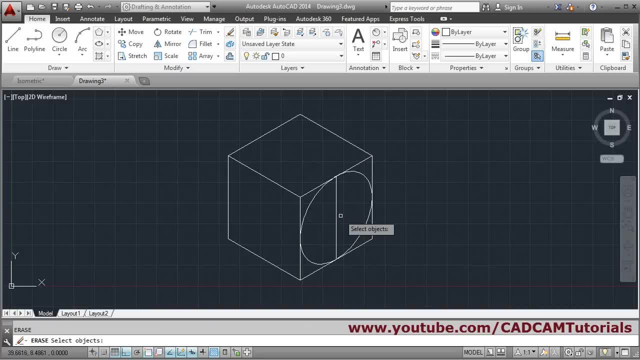 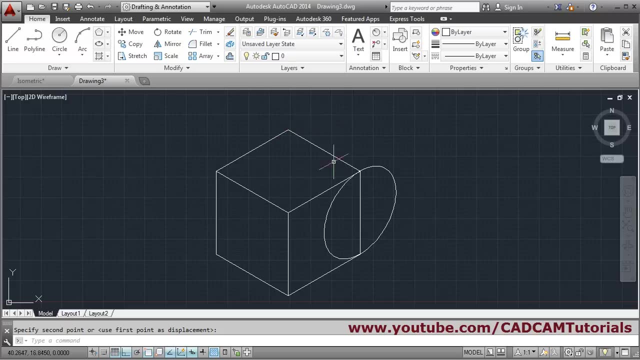 created. suppose I want to create circle here. so I will just erase this and move this. select object: enter. so I want the center of this circle at this intersection. suppose I want here portion like this, here also I want circle on this side also, so I will just copy the circle. copy: select object enter. take. 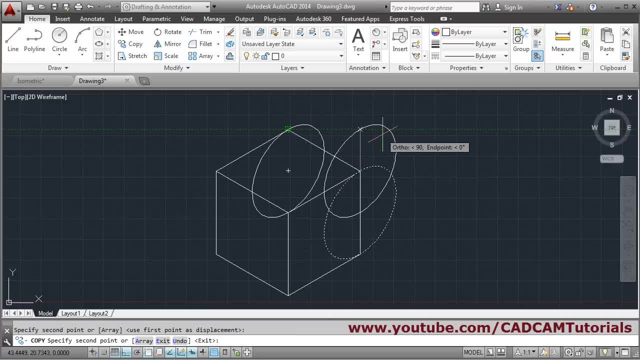 this intersection point. and second point will be this intersection point. this is my selection point. you can see a circle and here is the point. so I section, press enter to come out. then i will need to create one line here. so just take line command and you have to choose the quadrant option. don't go for tangent, go for quadrant. so you have to. 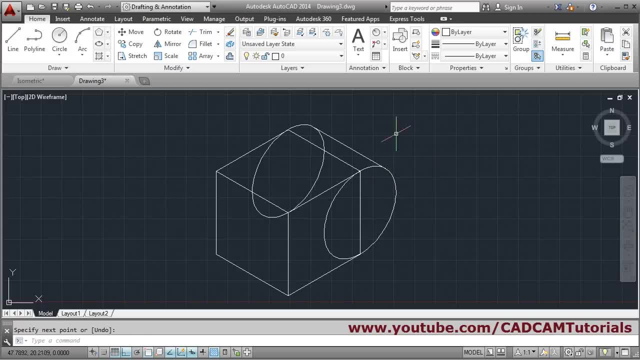 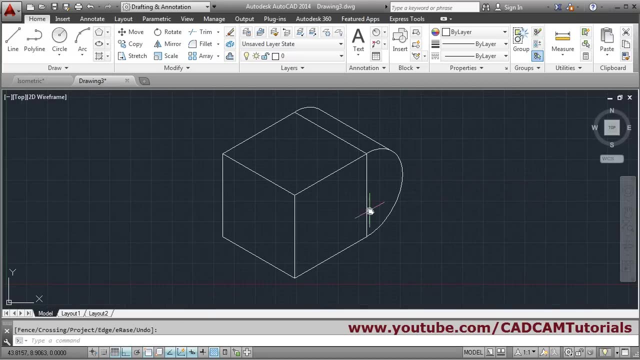 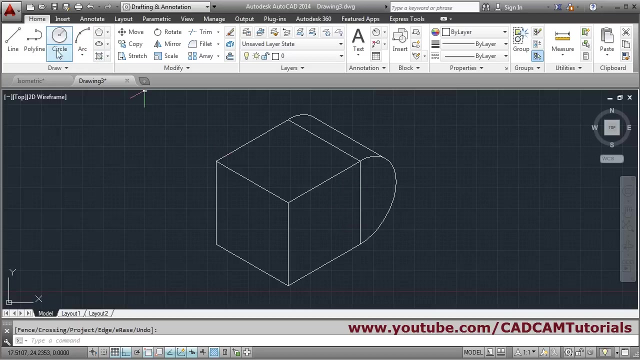 connect the quadrant points, then press enter. then unwanted portion: you can trim it. trim, select cutting edges, then press enter and click on the non desired objects and press enter. so in this way this portion is created again. suppose i want a circle in the center here? so again i will say: 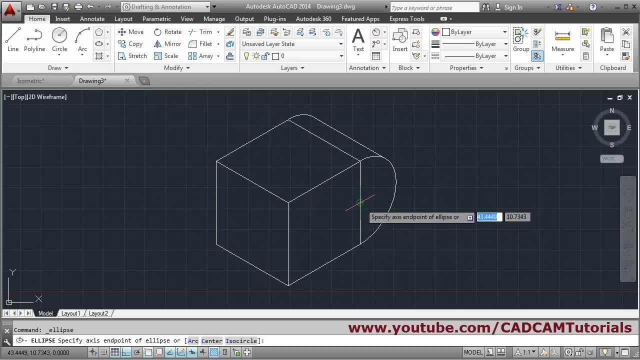 ellipse axis end, then give the center point. okay, don't give center point, ellipse axis end, you have to click on iso circle. so then give the center point and give the radius how much you want. suppose i want 2.5. so in this way you can create that radius. so if i don't want this center line i can erase it. so in this way this: 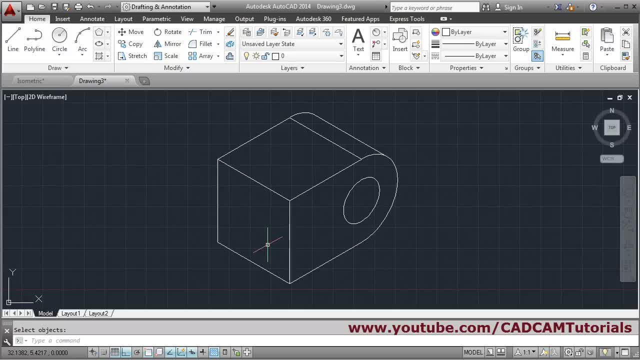 object is created and to give the dimension for this object you have to use aligned option. so click on aligned, click on the first first point, then center point and give the radius how much you want. suppose i want 2.5. so in this way you can. 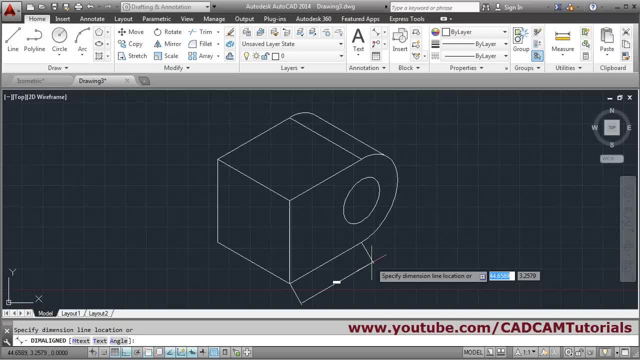 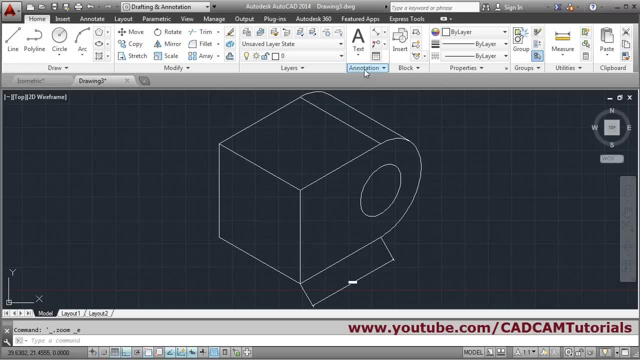 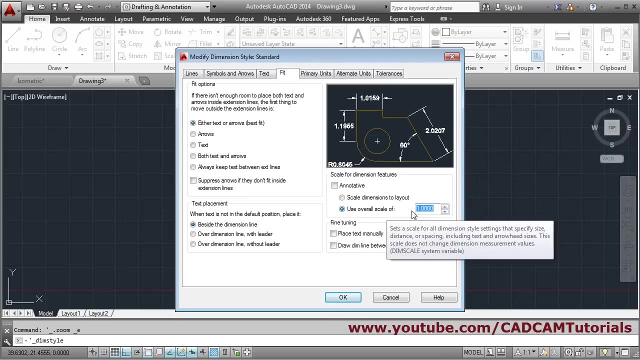 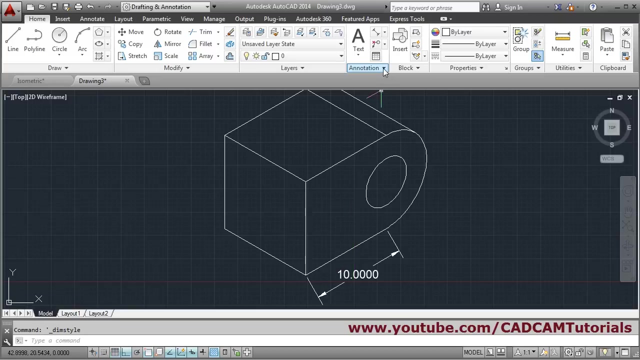 give the second point and give the location. so here dimension is not properly visible. just take annotation, dimension style modify, fit and increase the scale to suppose 5. okay, close, so it is properly visible and you can also control the other settings, modify then. we don't want the. 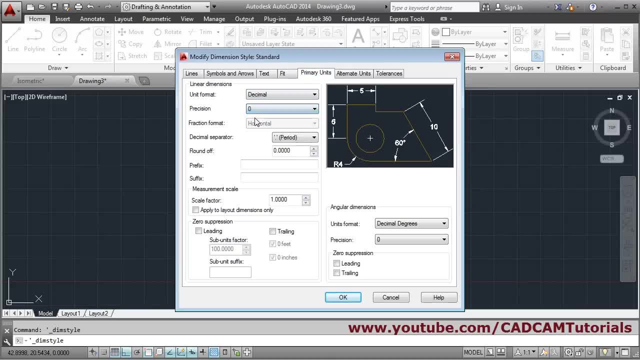 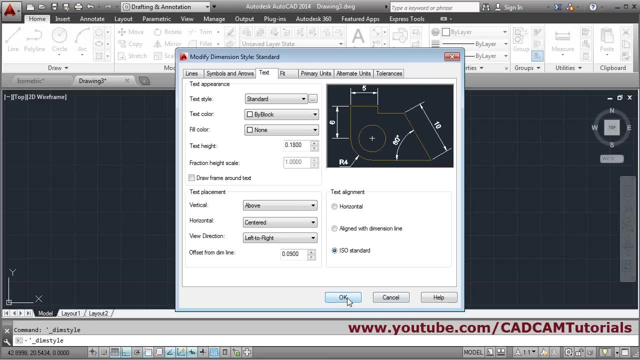 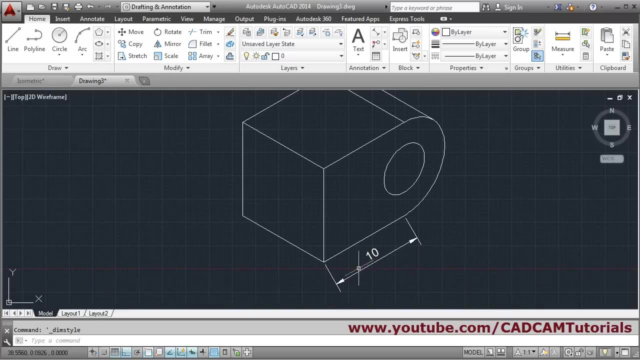 you can also control the other settings, modify then. we don't want the precision to four digit, i want single digit. again, text: i want it above, so it will come above, and i want iso standard. okay, close. so in this way this dimension will be properly visible. then now this: 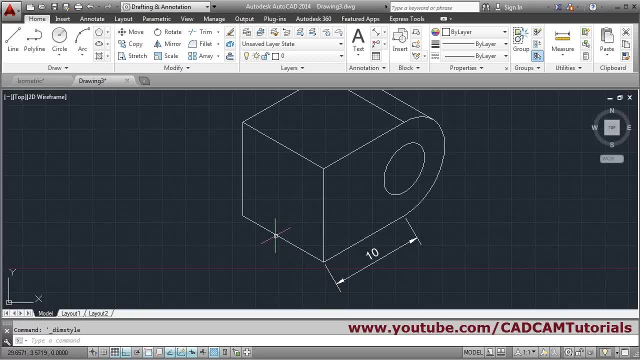 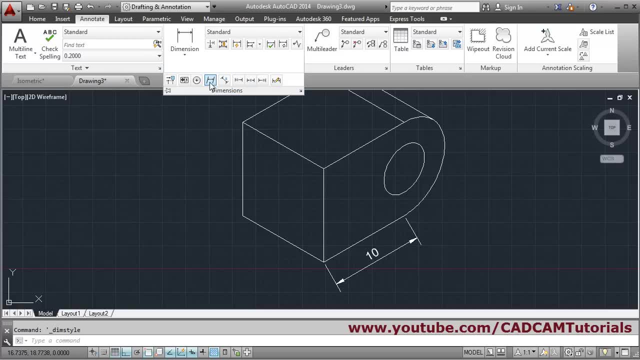 dimension is not coming properly. it is going downward, so i want it to be aligned to this line. so for that you have to go to annotate, click on dimensions and select this oblique option- oblique, then select object, enter, then enter oblique angle. so angle of this line is 150 degree. so 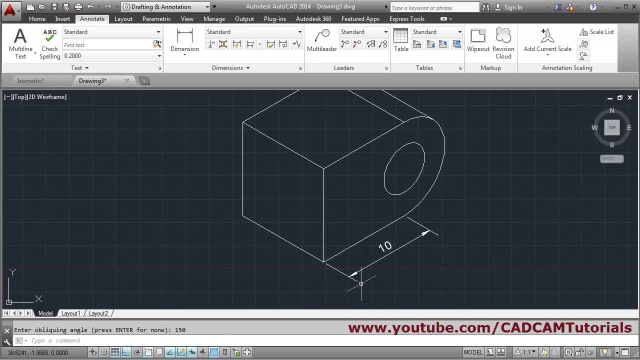 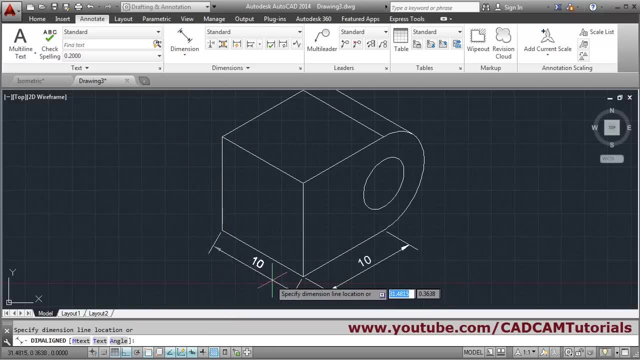 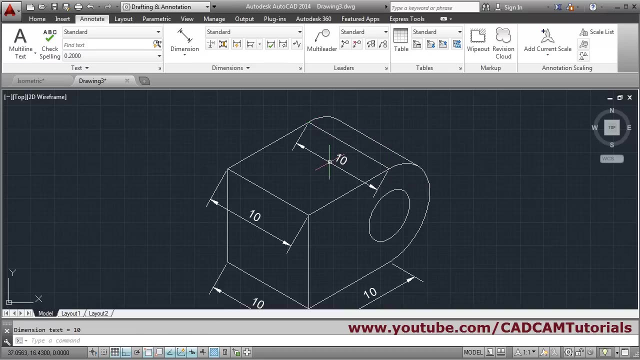 we'll just give 150 press enter so it will properly align to that line. so again, we will give some dimension using aligned suppose. here i will give it press enter to repeat the dimension command. we'll just take some trials. again i will go for dimensions oblique. 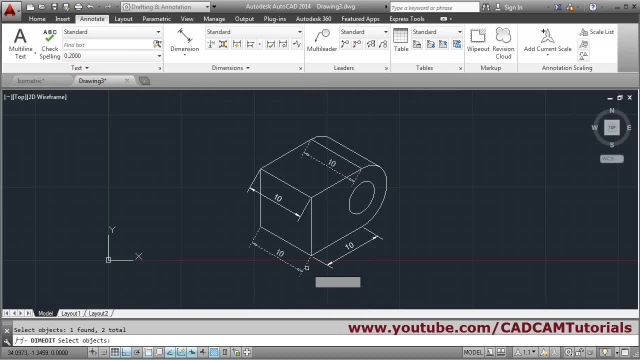 then select this: two dimensions. so this dimension i want to be aligned with this line. so you have to pay the attention to the extension line, not to the dimension line. so you have to align the extension line. so this line angle of this line is 30 degree. so we will give select object, press enter. we will. 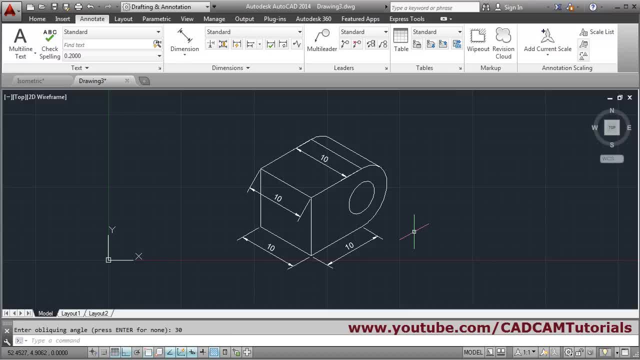 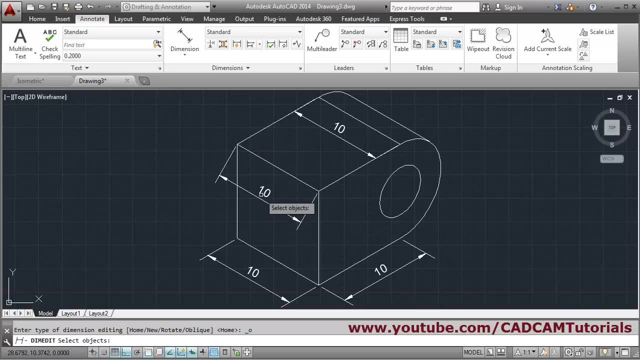 give oblique in angle as 30 enter, so in this way it has been aligned properly. then next again for oblique select object: enter, then oblique angle. i want it to make vertical, so i will give 90 degree, so in this way it has been. 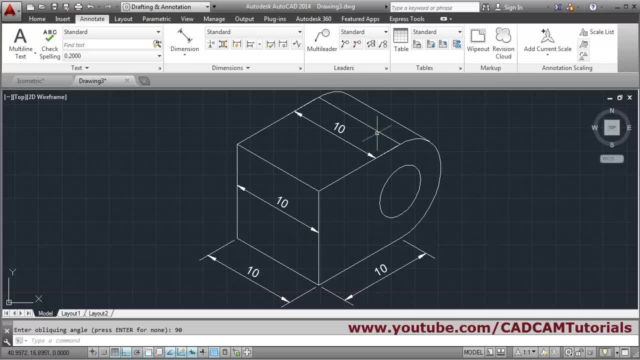 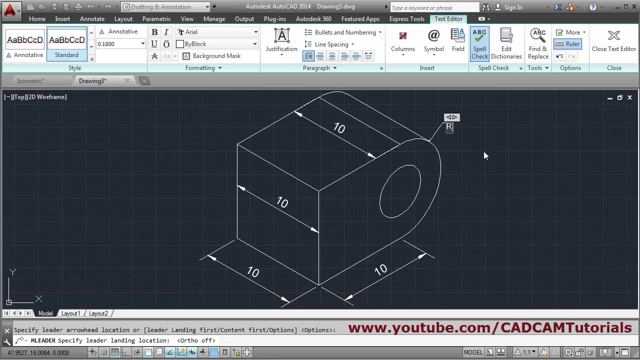 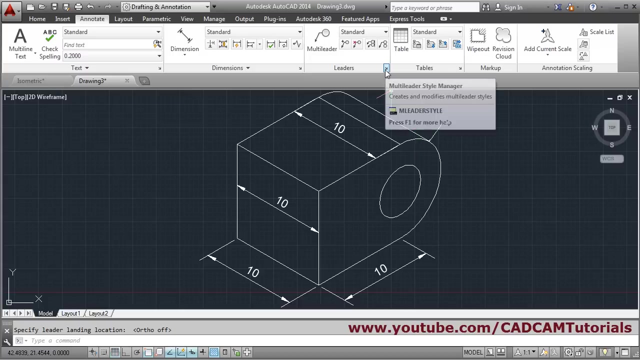 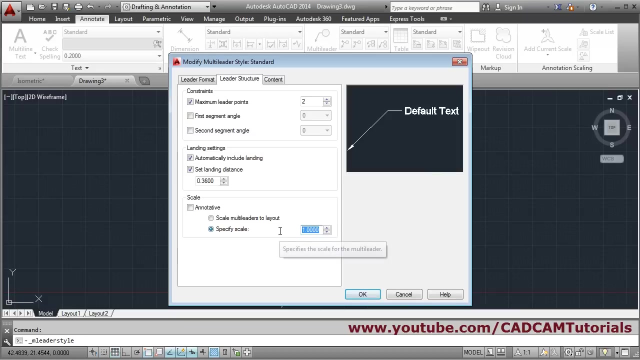 properly dimension. then for circular part i can use the multileader, then click on the end point or quadrant point, then make ortho of click and give the radius what is radius for you. click outside. so now it is not properly visible. so from here: multileader style. click on the multileader style. modify leader structure. specify scale. increase the scale to.